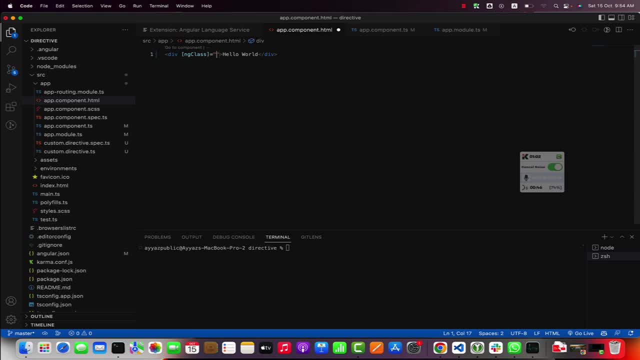 There are many more directive like ng class, So these are the examples of the built-in Angular directives. So in this video we are going to build a custom directive from scratch. So this would be very easy and straightforward process. So I will explain everything. So right now you can see that. 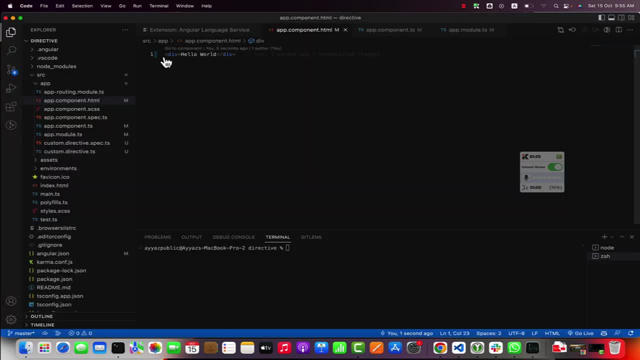 I have this very basic Angular div, So this is HTML div and I have some text in it. Now I'm going to generate a custom directive, So let's generate it. To generate Angular directive, you have to run this command: ng generate directive. 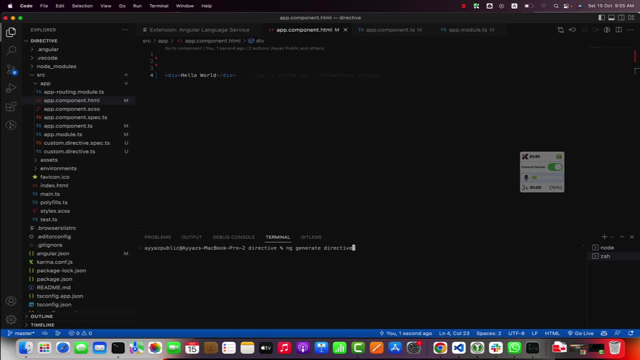 And obviously you should have the Angular CLI installed already in your system. then this command will work. So I am writing ng generate directive space And then you will write the name of the directive that you want to generate And then you will write the name of the directive. 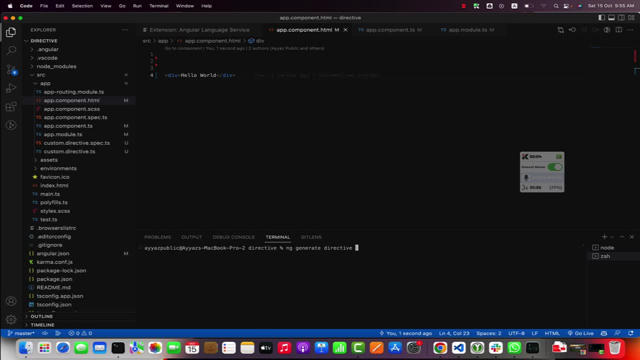 that you want to create. So I want to create a directive, for example. I wouldn't, you can name it anything. I'm going to name it, change me Okay. And I want to place it inside a different folder. For example, I want to put it in the shared directive slash. change me, and this in this. 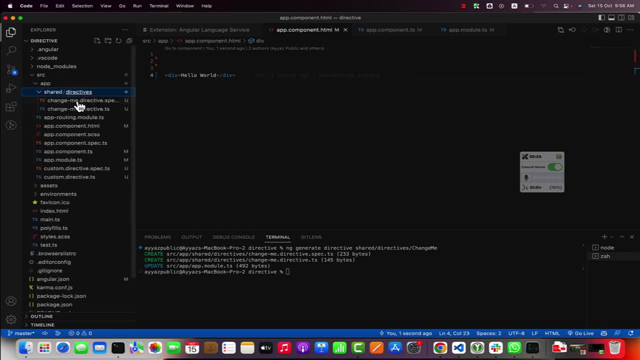 way, it will create these folders for you, like shared directives, and it has created this directory for us. So, and you can see that these files have been generated. And also it has updated our app module. if you go to the app module, then you will notice that this directive has been declared in this: 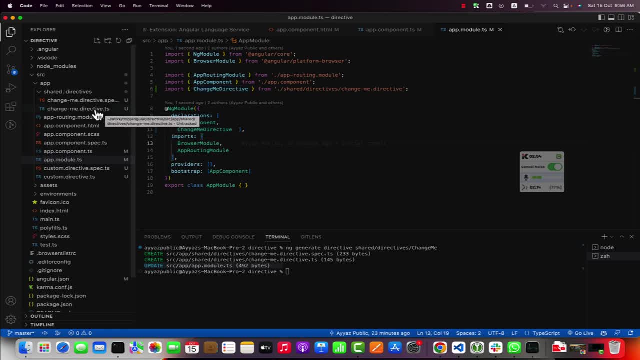 module automatically. you did not have to do anything After that. if you go to this directive that you just generated here, you will see that this is a very basic and simple class without any code in it, And you can see that it also has added a selector for you, So you can use this. 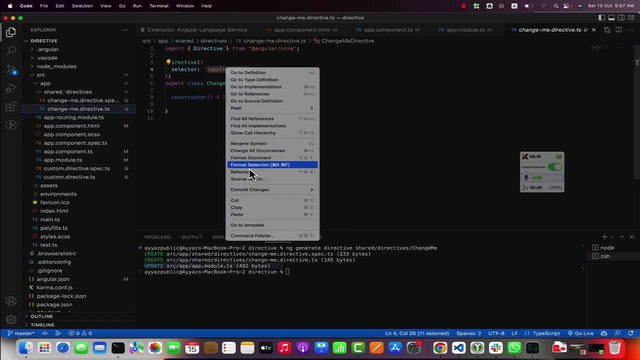 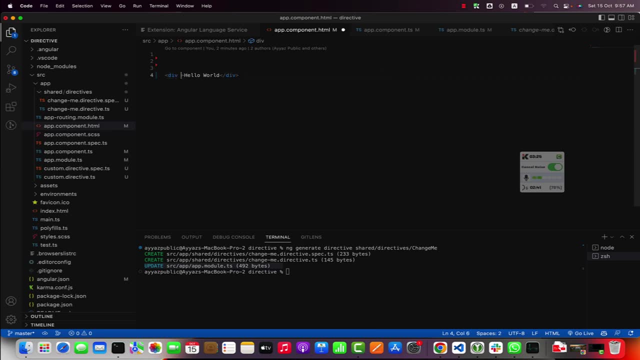 selector to element. for example, let's copy this name and go back to your appcomponenthtml And here you just have to add that selector like this, And as soon as you add it it will start doing its magic. So let's go back to the directive, And in this directive I am going to inject the element. 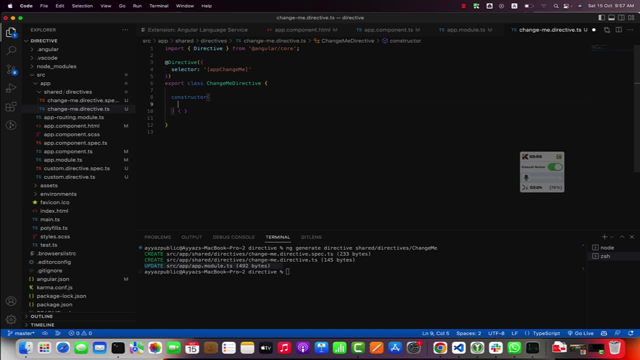 reference. So with the help of that, I would have access to this HTML element where I have added this directive. Okay, so just add private element, element ref. So when you are typing in the VS code it actually shows you some suggestions. So, for example, I'm typing: 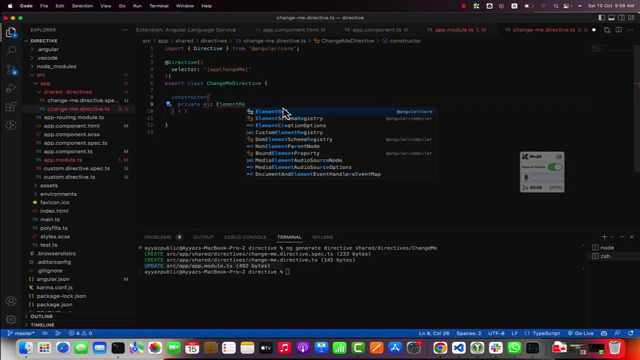 it. So you can see that it is showing me this suggestion that you can import it from here. if you click on that or if you press enter, then this will automatically import that library for you. So this would be useful for you if you don't know about that. Now we have injected this element. 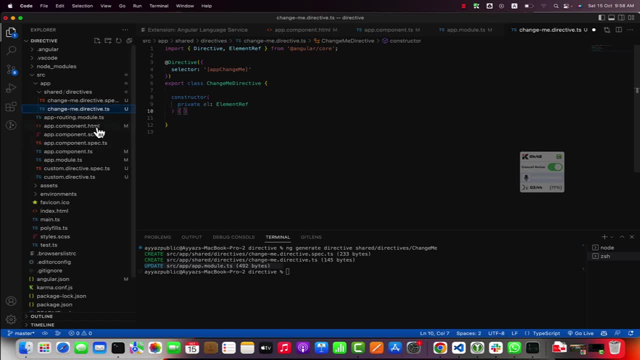 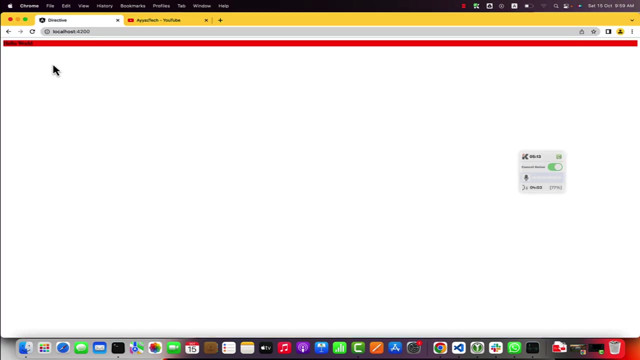 reference into this constructor. So now we can have access to that HTML element And then we can make changes to that element. Let's try to make some changes. for example, So if you type this dot element, dot, native element, dot style, dot. background color red, then if you 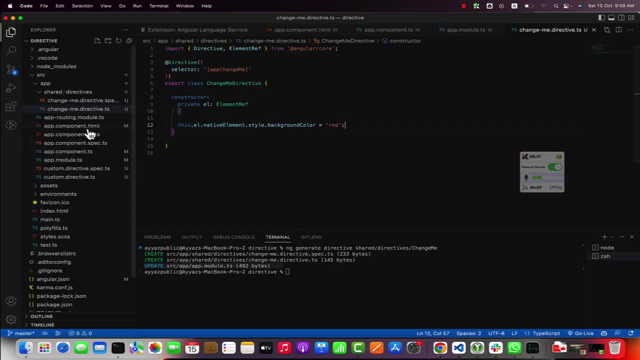 reload it, you will see that the red color has been added. I will show you again. if you look at here, we did not add any styling. I did not add any styles. Okay, I just added this directive and I added those. 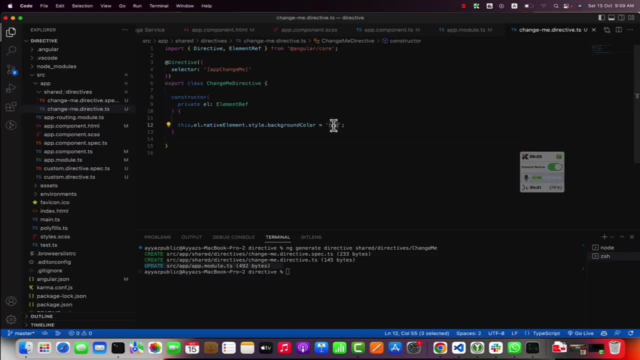 styles with the help of the directive And you can see that it is being applied. If I make any change, for example, I add yellow, then you will see that the background is yellow now. So, similarly, you can add multiple styles if you want. For example: 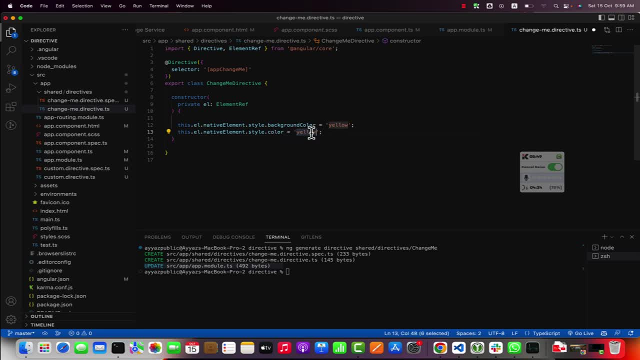 if you want to change the color of the text, then you can just add style dot. It is very simple And it is the same thing like you do in the JavaScript. So here in the native element you have the DOM element, And now, if you get the DOM element in the JavaScript, you can easily 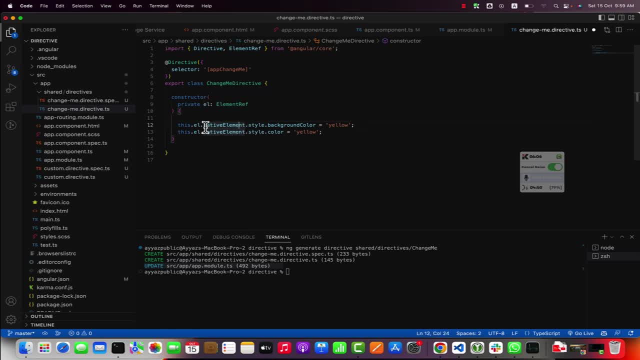 manipulate that element You can easily style. So after this part everything is same, like in JavaScript. So if you know JavaScript- how to customize a DOM element- then you can do this as well. So I changed the color to black. Let's see, It was already black, so I will try blue. 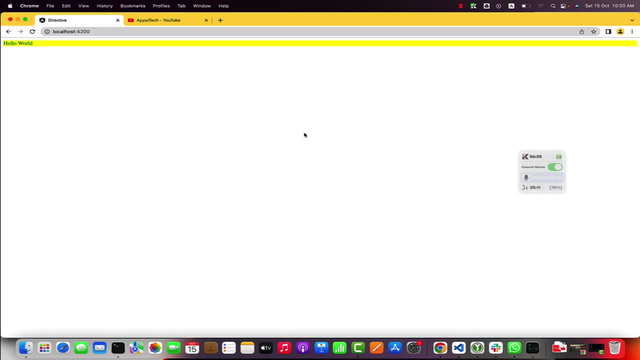 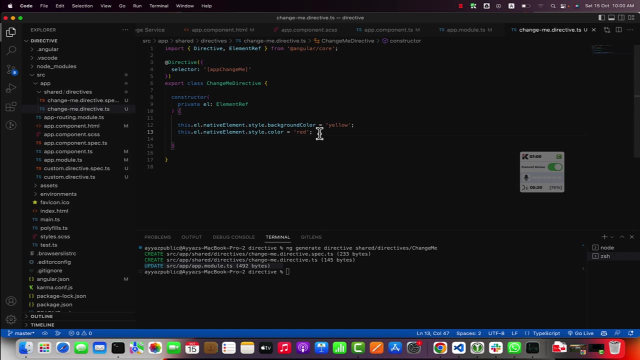 Okay, let's try some more visible color- Green, I guess. Okay, you can see that background is also changed and the color is also changed. If you want to add some text in the element, then you can do that as well. 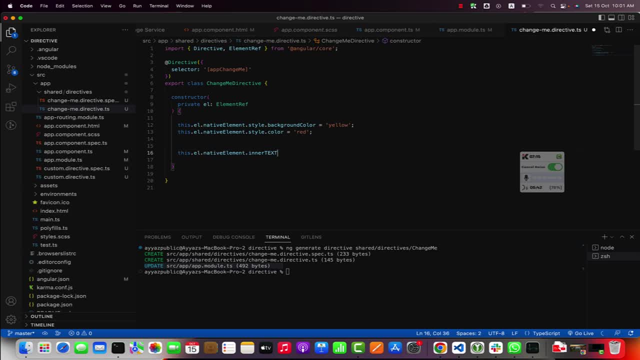 For example, this dot element: dot. native element: dot. inner text is equal to: I am changed. Okay, You can see that it is being applied. It is not replacing it, It is just adding. So if you add inner text here, you will notice that it will be prepended. It will be added in the beginning of. 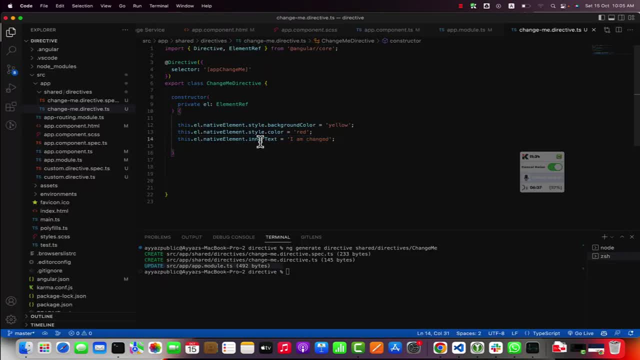 the text. So this is how you can add a text By using inner text. So the last thing I would like to show you that you can also add inputs at here. For example, if I add input, Input My name, Okay. 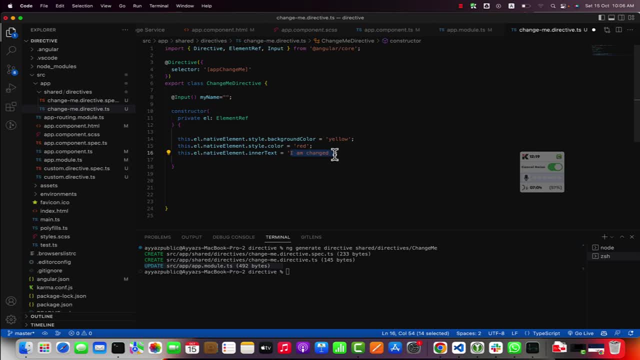 So if I have something in this variable, I will add it in this area. Okay, So right now you can see that nothing is being added inside and some things are added outside. Of course, the key: this shows that everything is in the element. I am seeing someornate open this. new this text. So its home sectionAngle, as I show it, is complete, So I want to click on this And in this upper finger I can also drag it down or drag it on. It is my home. Okay, So the right side, the dot column I am set to here. So for input name I am also señel einmal. 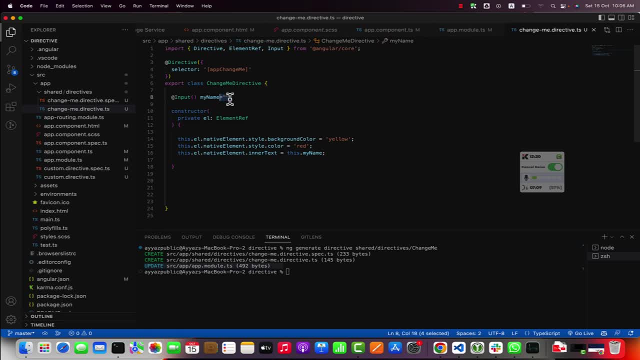 And this is how it really works. I am just going to roll over to do like the direct entering. so right now you can see that nothing is being shown here because by default the value is empty and if you go back to the HTML, then you can provide that input.